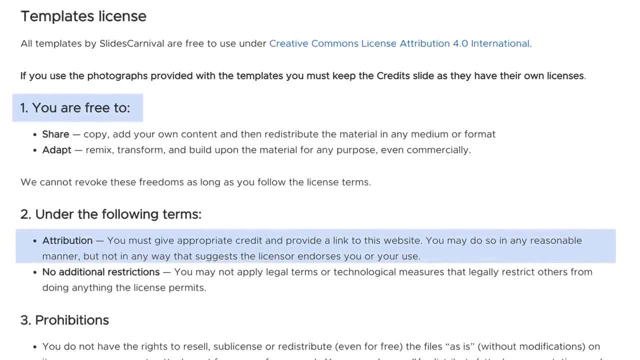 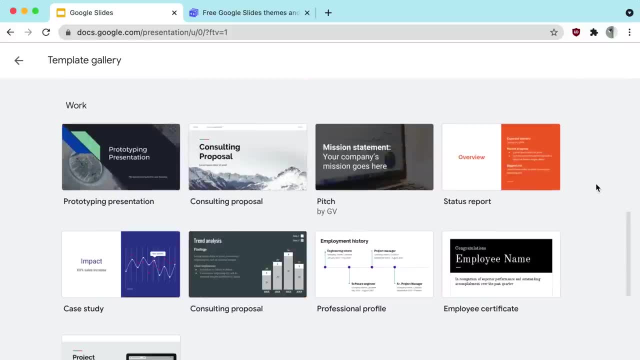 the templates are available for both personal and commercial use. Alternatively, you can also check out the template gallery that comes with Google Slides or slidesgocom, but they both have a few limitations. The template gallery doesn't have that many options and slidesgocom limits your download. 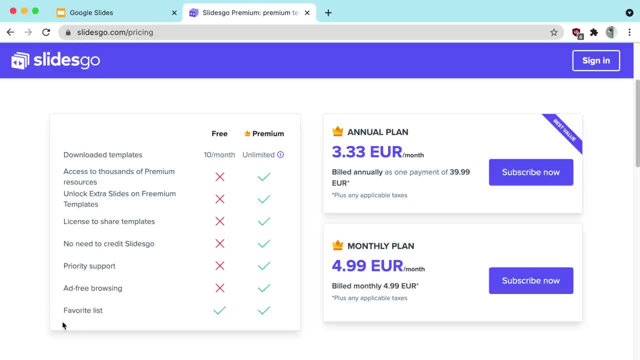 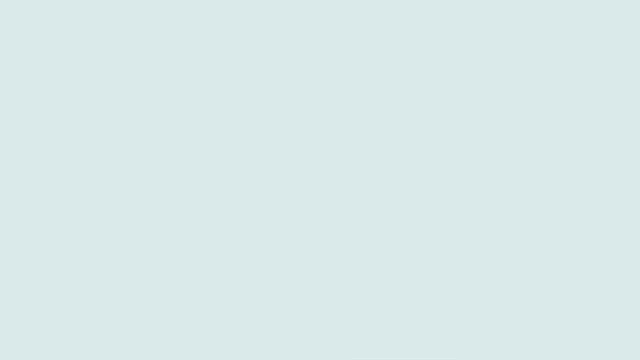 to 10 free templates a month. Any more than that, you gotta pay and go premium. Now that you have a great template, you wanna customize it and make it your own, And this is where websites like colorhuntco comes in. I use this tool to pick a color palette. 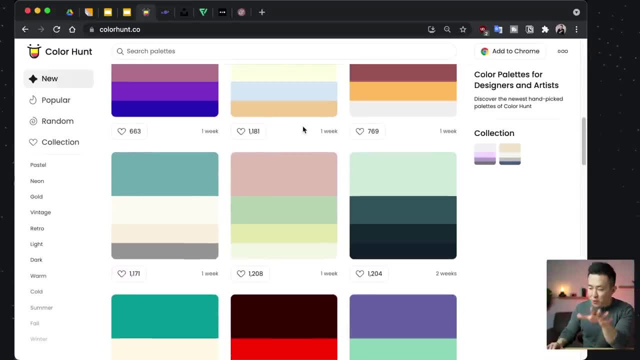 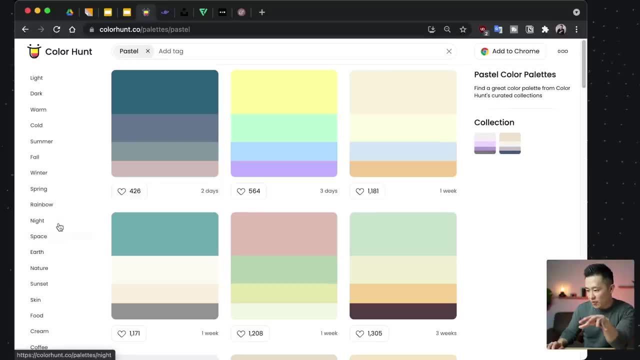 that I will apply throughout my entire presentation. I usually take a few minutes to browse the popular pastel and night categories all the way down over here. By the way, I'm almost positive like this is the MKBHD branding. 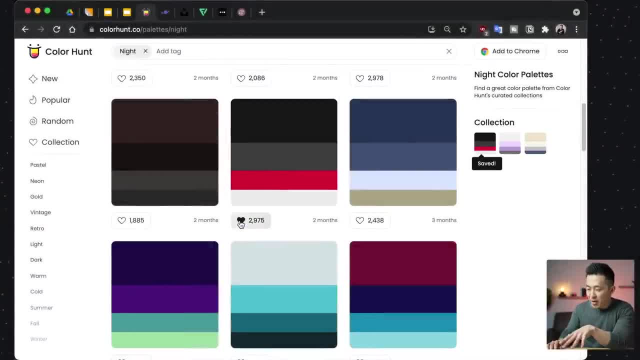 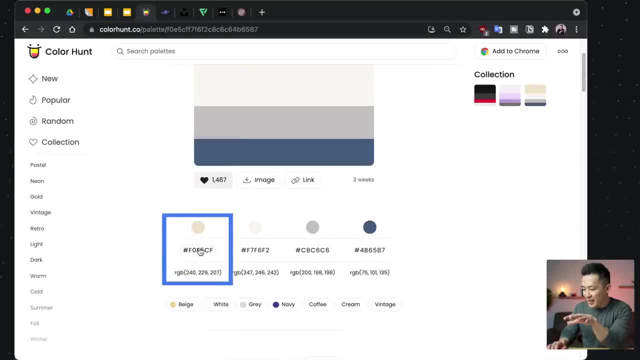 I'm not sure. maybe one of you can let me know And I would favorite the ones I really like and it gets added over here. Then when I'm ready to apply the color palette, I click into it. click on the hex code. 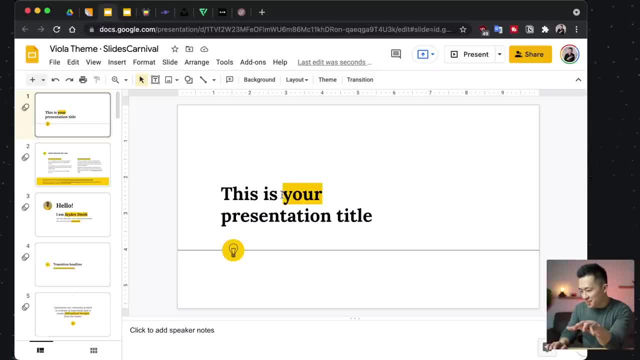 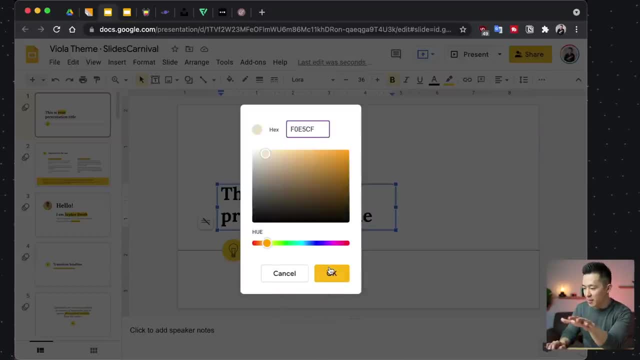 to copy it to my clipboard. go back to my presentation. select the color I want to replace by clicking the highlight color here, adding a custom color, pasting the hex code in, pressing okay. And for elements you can't seem to click on. 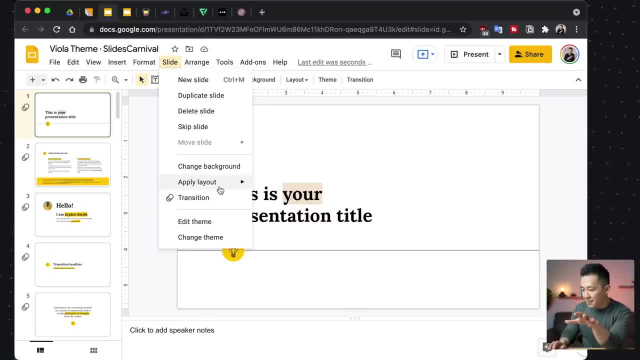 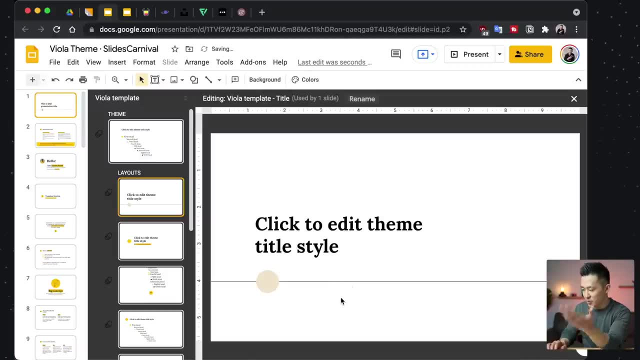 like this one right here. all you gotta do is go to slide edit theme, click it here, change the color by again choosing the color you just added, clicking X to exit out. Look at that. I just made this template unique to me. 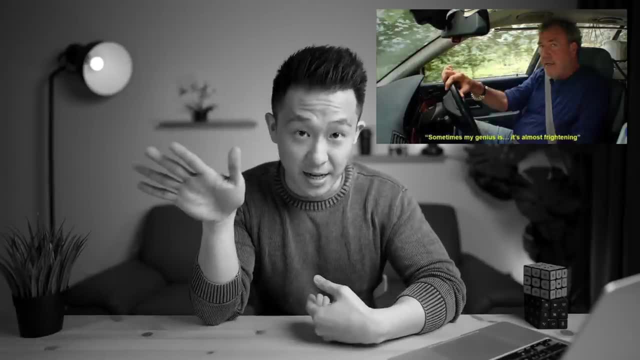 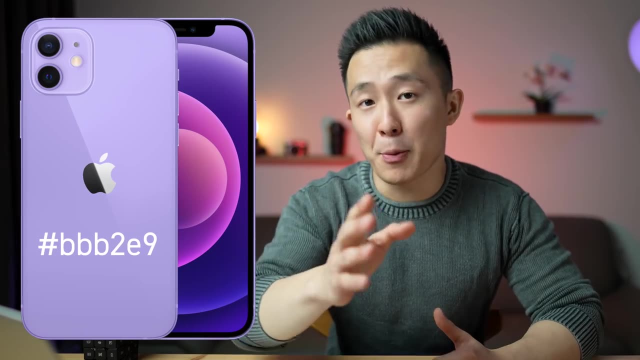 I'm telling you, sometimes my genius is almost like frightening. Okay, but what if there's one color you really like and you wanna build around that dominant color? Let's take the totally not a scam purple iPhone, the hex code of which I'll throw on screen right now. 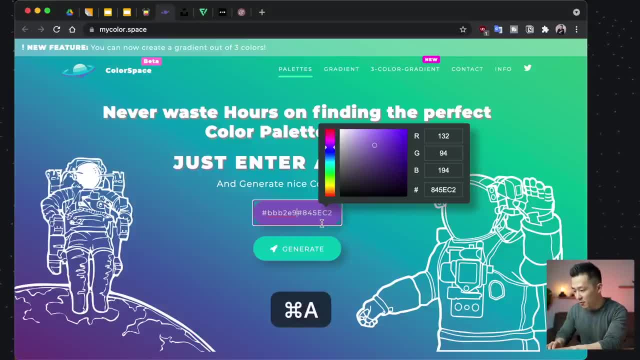 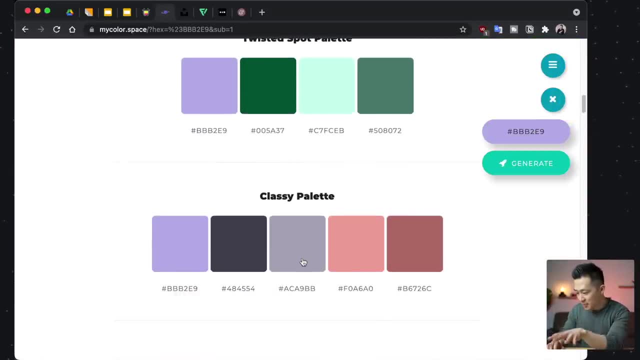 If I input that into a website called color space, like so, it can generate a bunch of color palettes around that dominant color. For me personally, I usually go with the natural palette like this one, but there's so many options on here. 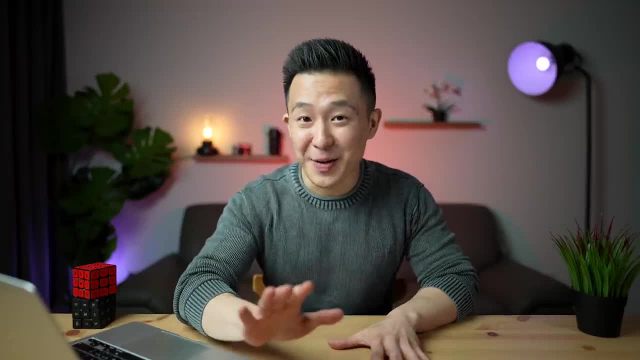 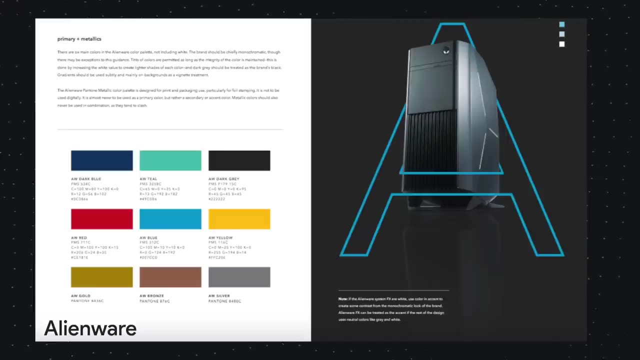 there's definitely something for everyone. Before you go crazy with these colors, by the way, most companies have brand guidelines in place for external presentations, but for internal presentations you can get a bit creative and show your personality. By the way, please do let me know. 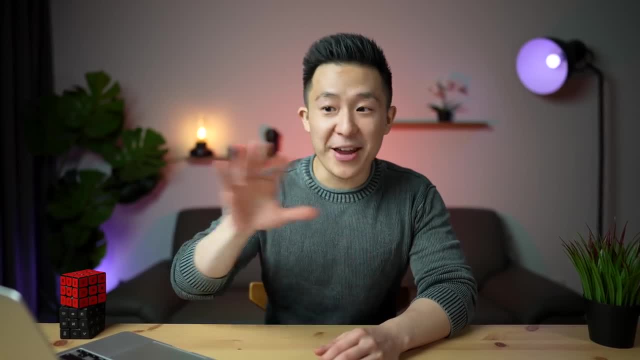 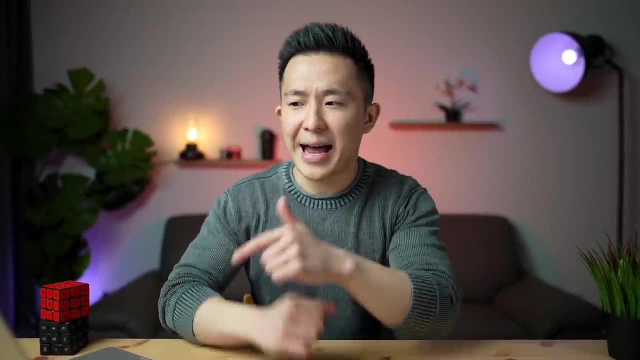 whether you're enjoying this Think Outside the Box episode. I have way more like work hacks like this, but I'm just not sure whether they're relevant for you, So let me know down in the comments if you wanna see more of how I use non-traditional tools. 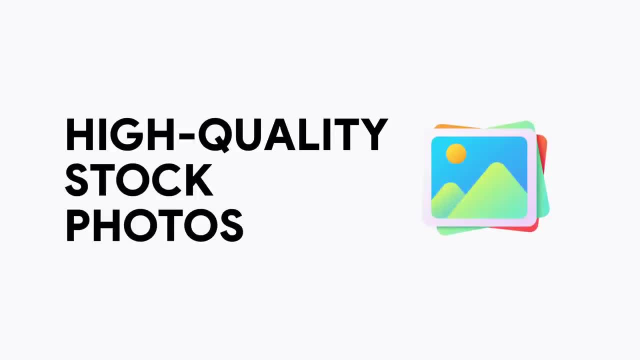 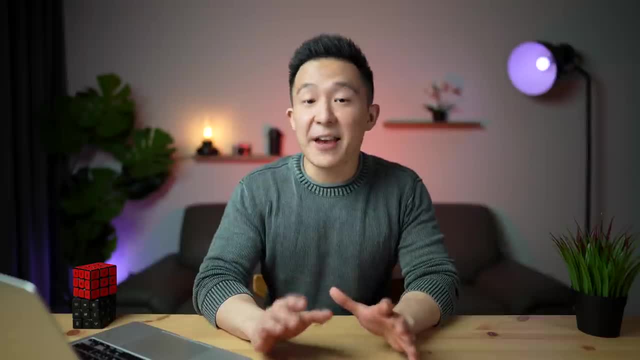 for traditional corporate work. Now you have a template and made it your own. it's time to add some images to help convey your message. Spoiler alert: we're not using Google Images. Instead for high resolution images, I use Unsplash. 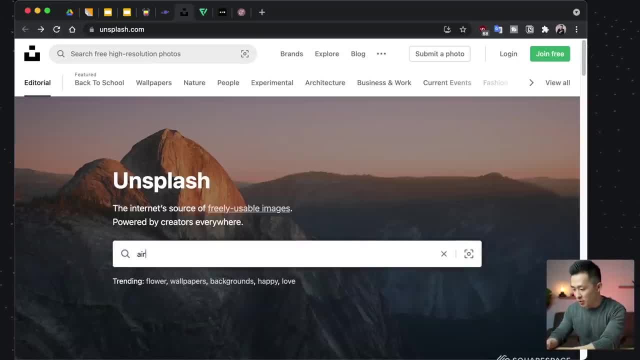 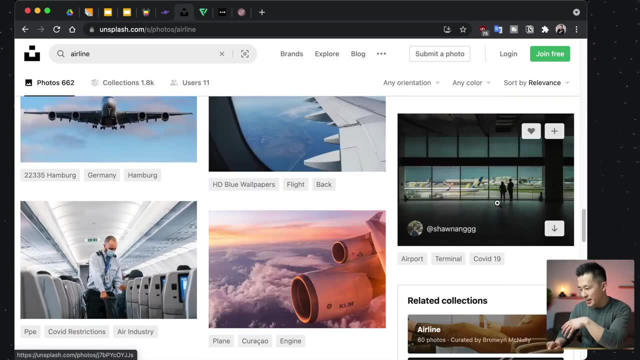 let's say I'm doing a presentation on airline travel. I type in airline in the search bar. here I go down and find an image that I think would be appropriate. Let's say this: one click, download for free. And going back to my presentation, 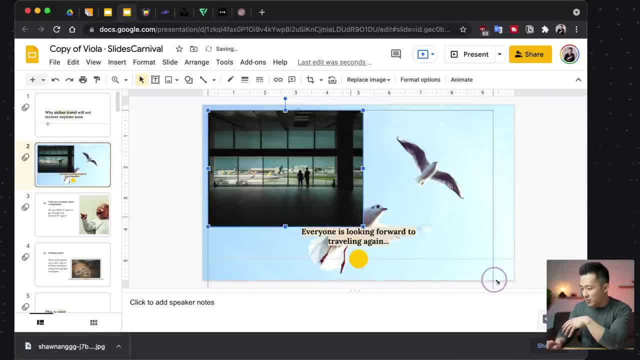 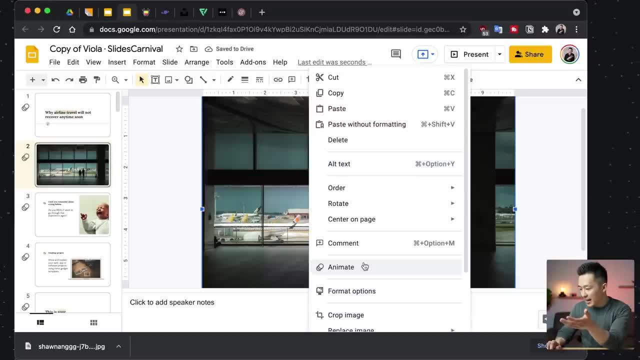 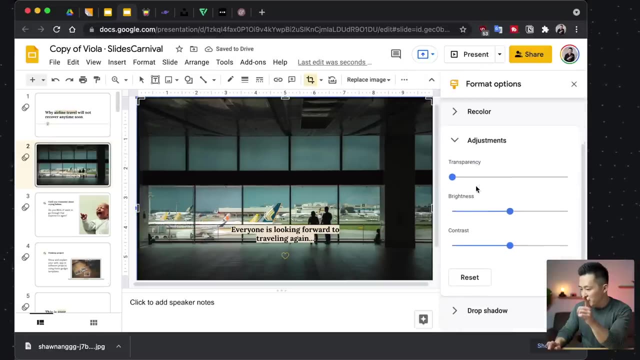 I drag this image into the slide, resize it a little bit to make sure it's covering the entire slide like, so I can crop it if I want. I would right click and actually bring this all the way back And pro tip and for under format options and adjustments. 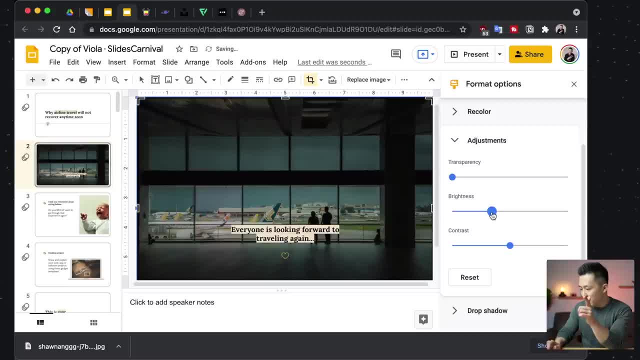 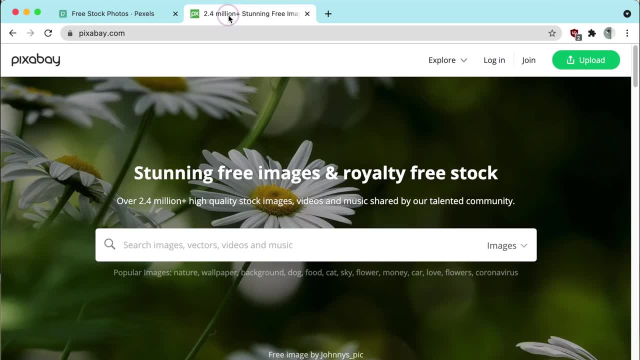 I actually like to bring the brightness down a little bit if this is a background image, to make the words pop out a little bit more. Alternatives to Unsplash include Pexelscom and Pixabaycom. They all have free, high quality stock photos you can use. 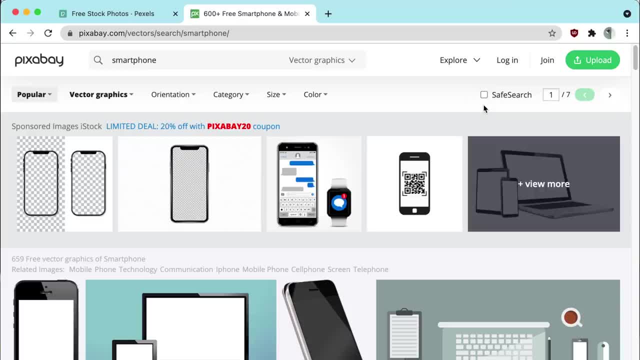 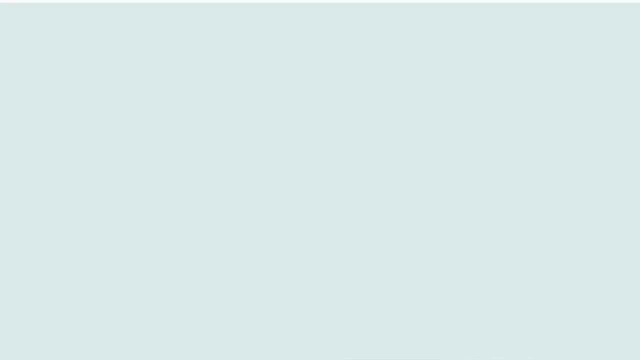 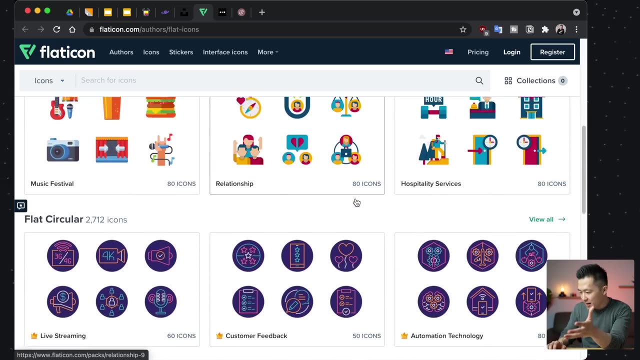 and Pixabay even has vector graphics similar to what you would find on Google Images, just in a much higher resolution, And most have a transparent background as well. And onto my personal favorite flat icon, Iconzcom. Again, I'm just amazed how many beautiful free icons. 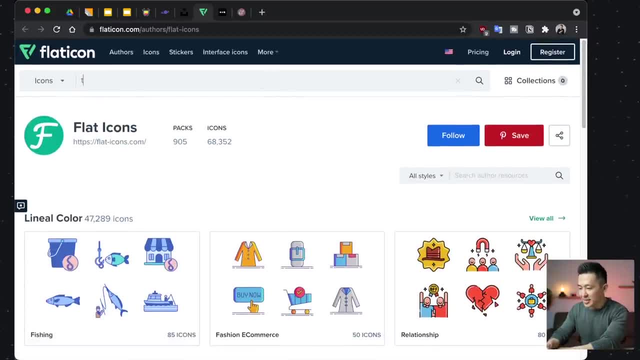 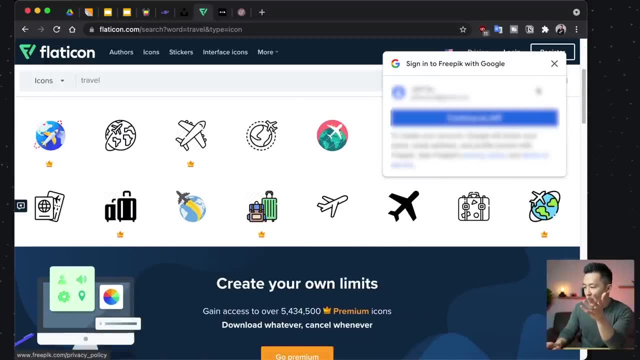 there are on this website. Back to my presentation. let's say I want an icon on travel, an airline- I just simply type that in. And the ones with the little crown on here are for premium users. you gotta pay, but there are plenty of free options as well. 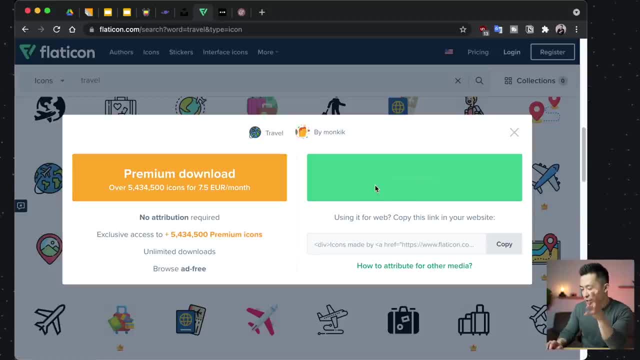 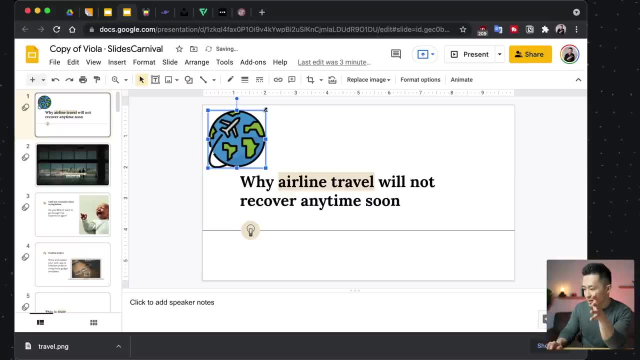 Let's pick this one. this looks pretty good. Free download. attribute the author, if you end up do using this. Going back to my presentation, here again, I just drag the icon onto the slide, resize it a little bit, and doesn't look too bad.